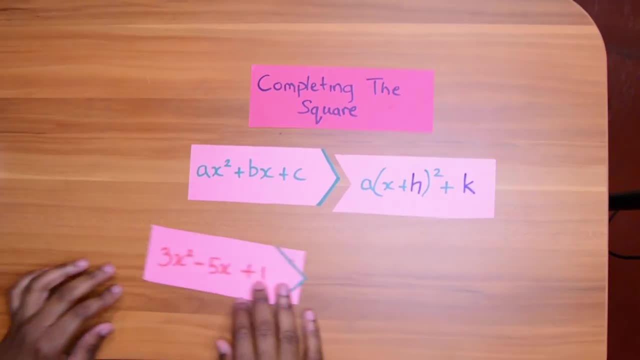 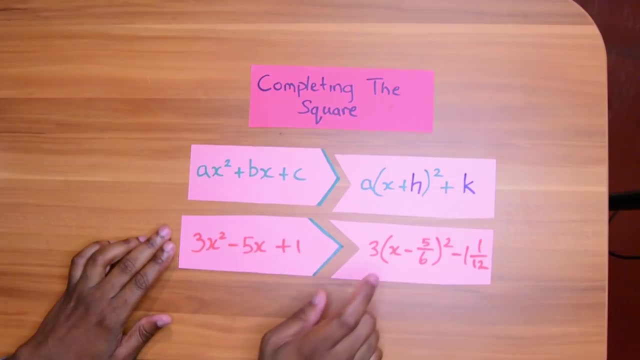 changing from this. look into this. look, For example, if we had this equation, this is a quadratic equation. We want to change it. This is the answer. We want to change it to look like this Now: wouldn't it be great if we had a formula for h? 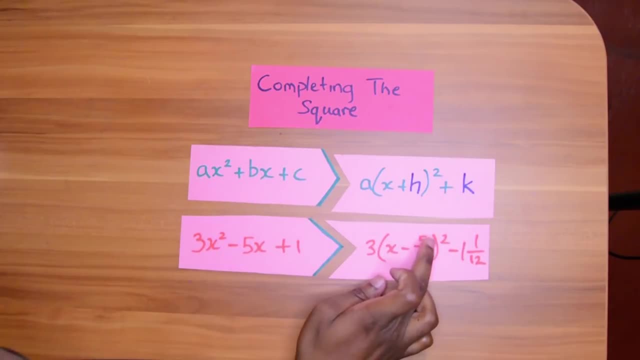 and k based on a, b and c, So like for negative 5 and 6.. If I could use these numbers to just get the answer one time, or to get the answer of a key one time in the example? Stay tuned, let me talk about this. 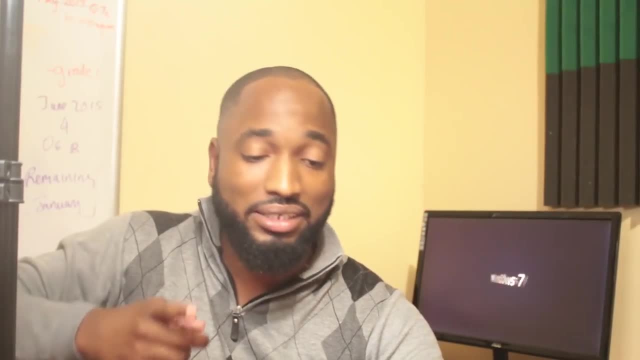 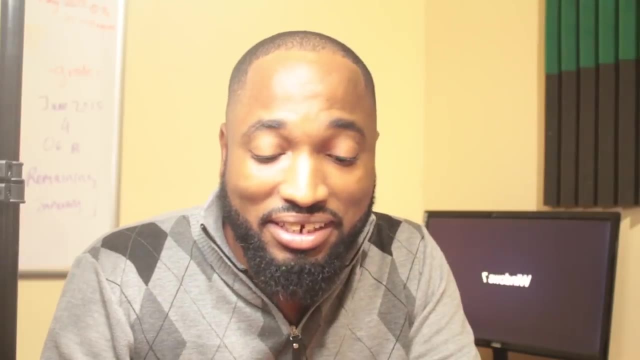 Now, one of the problems with completing the square is your teacher will show you one method. Your lesson teacher will come and show you the next method. Your cousin will come and show you the next method. I will come and show you the next method. You watch the next. 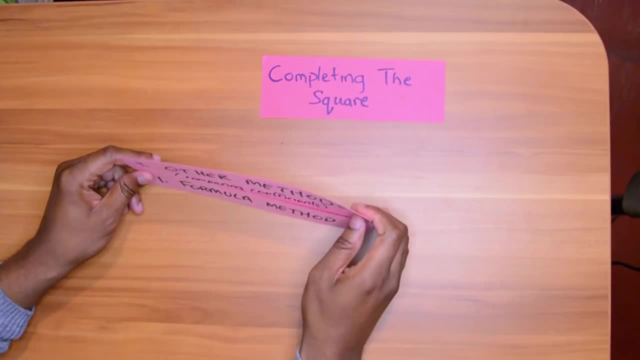 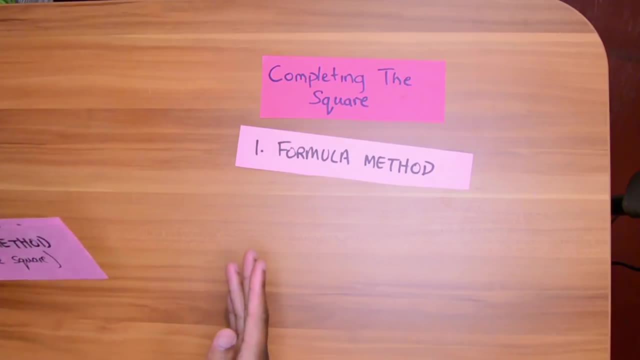 video on YouTube and see the next method. Then you go in your textbook and you say: next method: oh my gosh, What I'm going to talk about in this video is one: the formula method. Reason why you could use it, why you can't use it right, And we 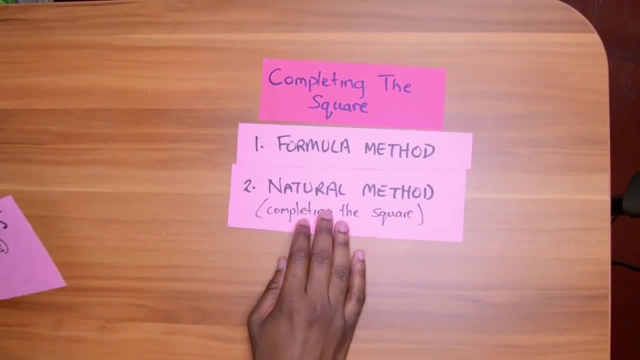 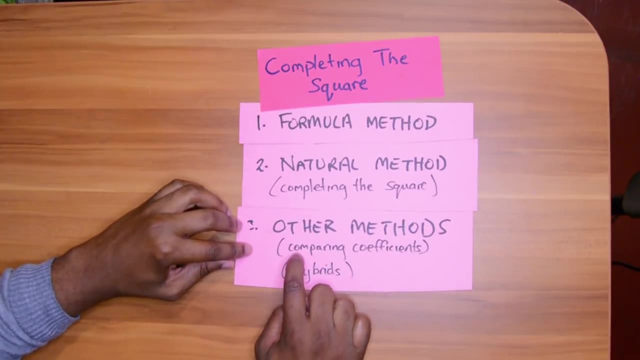 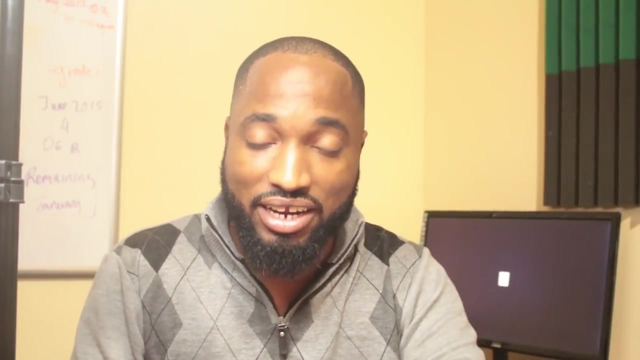 talk about the natural method, which is like the completing the square, the proper way method. This is my favorite method, And then we'll mention the other methods. The other methods are comparing coefficients and a hybrid method using maybe the formula method and the natural method together. Okay, we just mentioned. 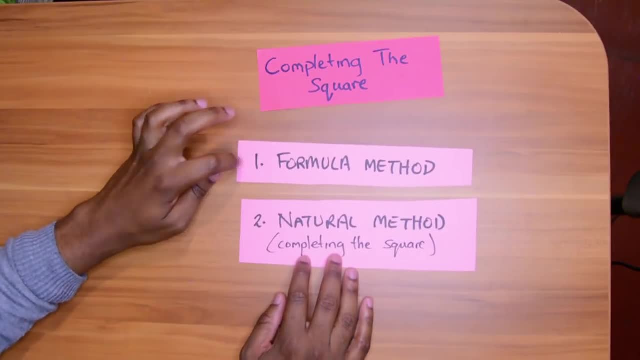 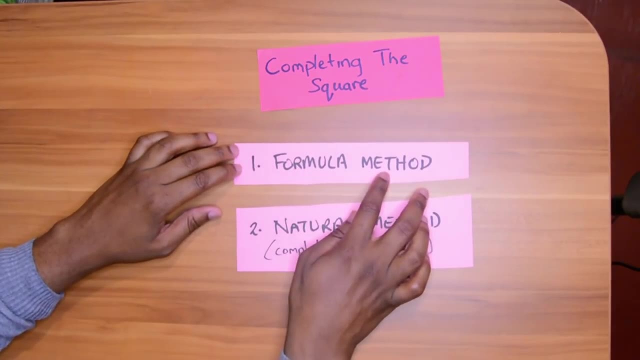 the other methods Right. so I would recommend that you learn this. but you try to do this. You try to actually complete the square. You learn the formula method just in case, because this is so easy. If you run into problems, at least you could complete the square and 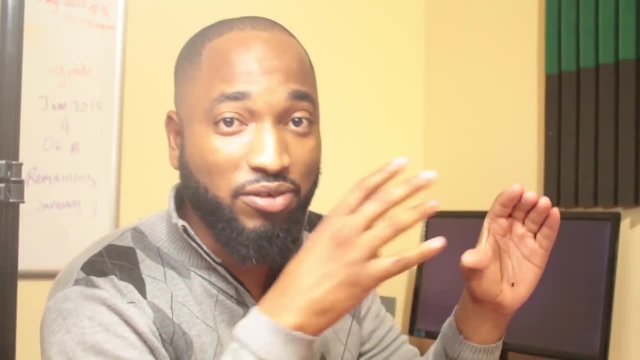 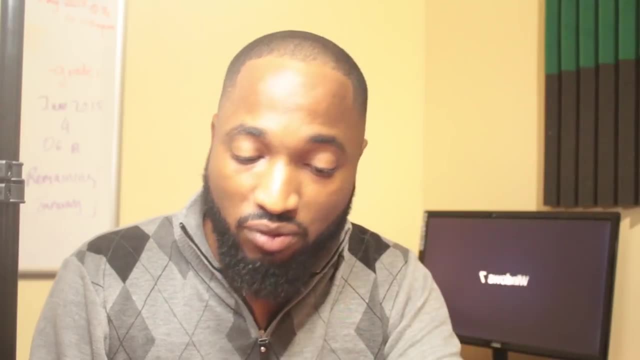 you want to always be able to complete the square, because after you complete the square you have to go on to get a whole heap of maths in the question. So you must be able to at least complete the square. And after you have quickly learned the formula method, try to 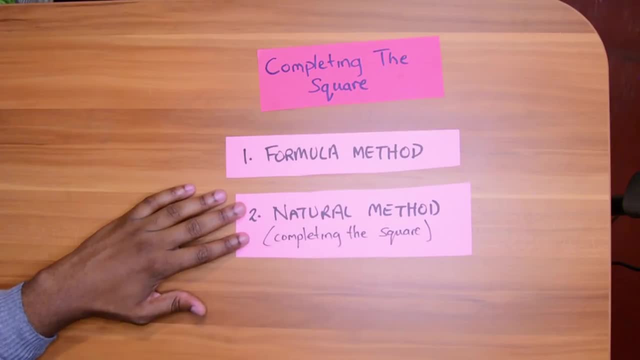 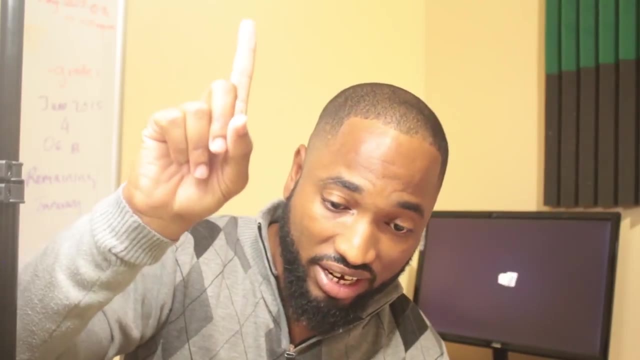 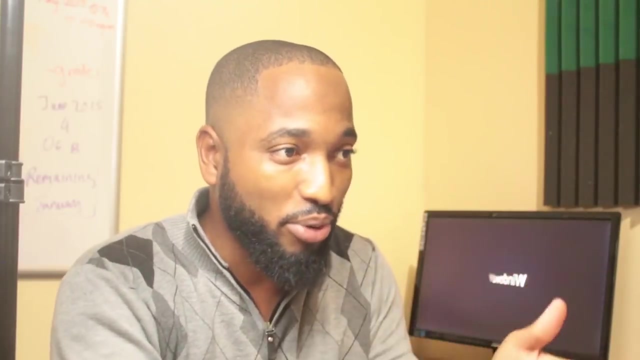 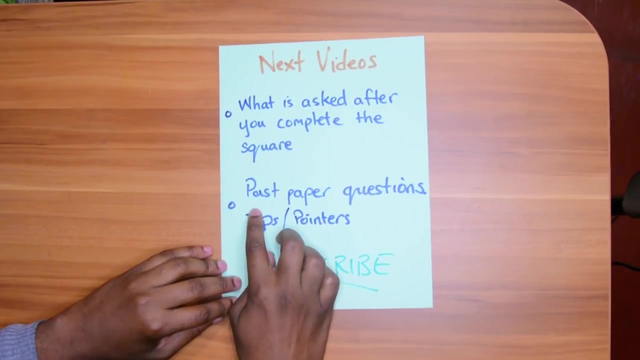 learn the natural completing the square method, Actually going about it. all these steps. Alright, let's go. Before I continue, what is next on this channel? Next videos: what is asked after you complete the square? After you complete the square, there's a heap of things you can ask. I will break it down into groups so you can see the three main things that they ask you after you complete the square. 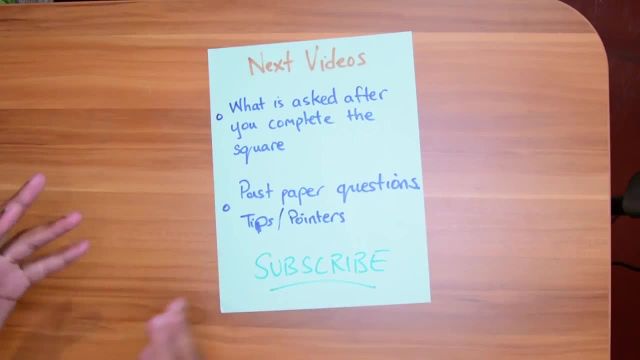 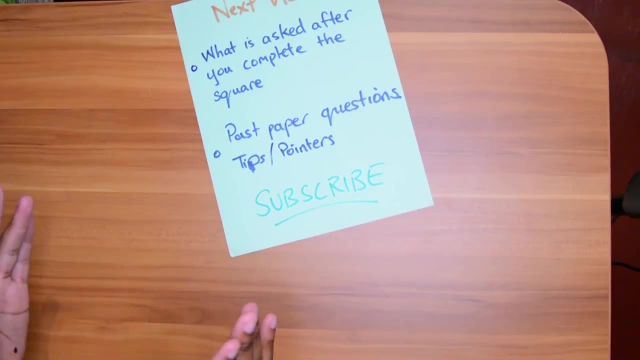 Past paper questions, tips and pointers, So maybe we'll do some. maybe this may be two videos, maybe it may be one, depending on how long it takes to edit And write. I don't remind people to subscribe enough, So subscribe. 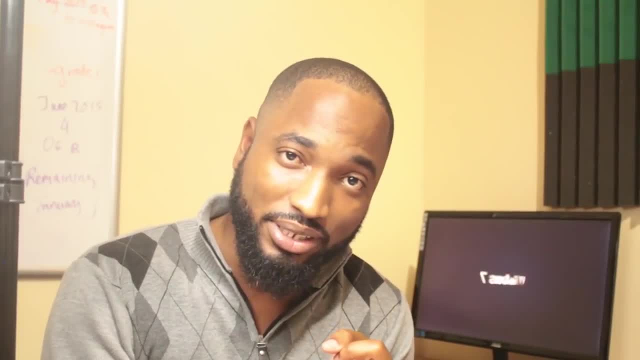 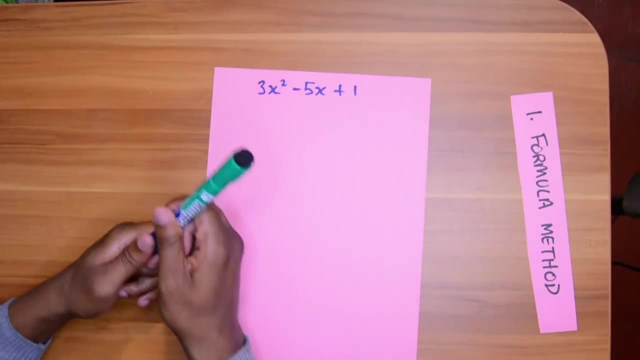 I post daily Maths and soon to be other topics, Motivation and just vibes. Alright, so let's start off with the formula method. This was a past paper question. Let's see if we can solve this Now. this is important. Everything that I do follow the exact statement. 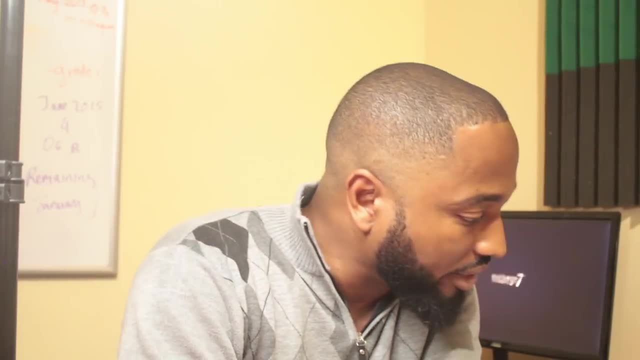 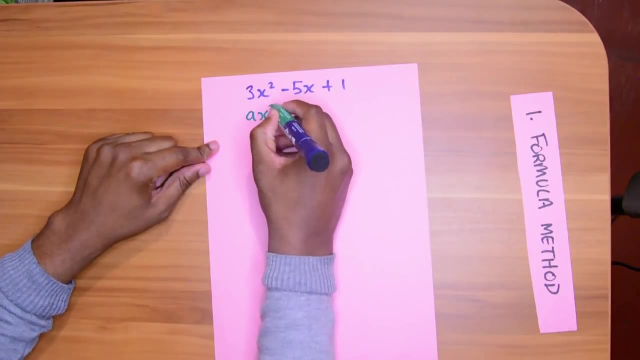 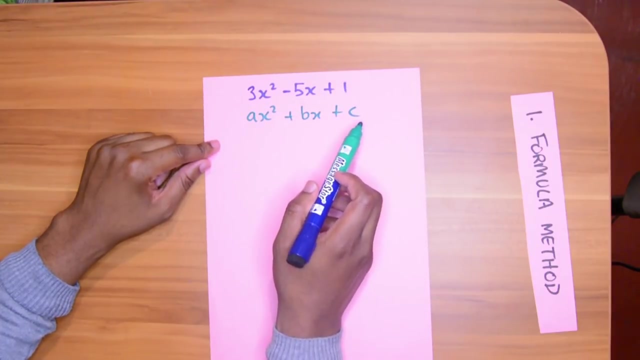 the exact settings. Right? Please listen to that. Alright. so the first thing you want to do is write AX squared plus BX plus C. AX squared plus BX plus C is the general form of a quadratic equation. B is negative five, C is one, A is three. So we're lining up. 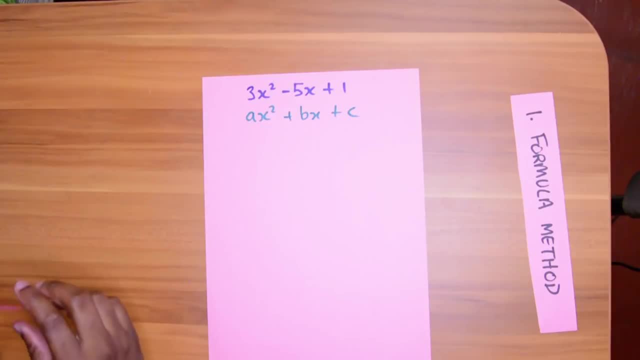 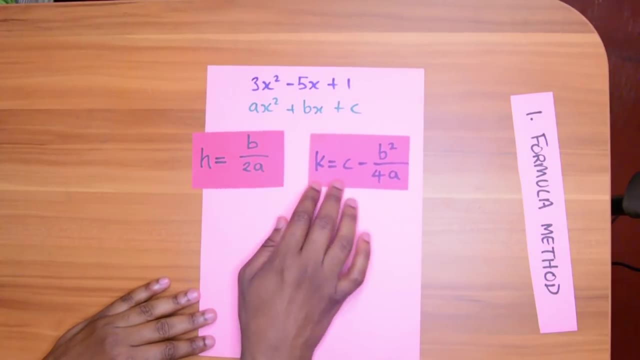 Because we're going to use a formula. The two formulas you're going to write next are these two guys: H is that B on 2 A and K is this C? take away B squared on 4 A. So So these are the two formulas you want to memorize. 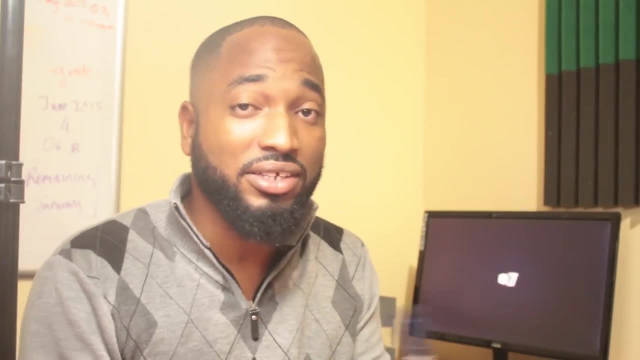 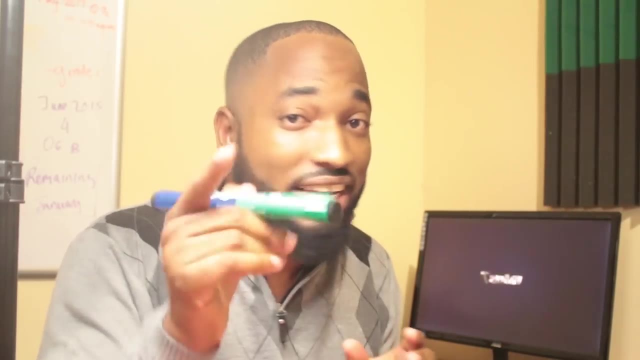 I would advise you right now: stop the video, write down the formula, try to memorize it. turn over the page, check yourself that you know it. write it down and at the end of the video, check and see if you know the formula again. 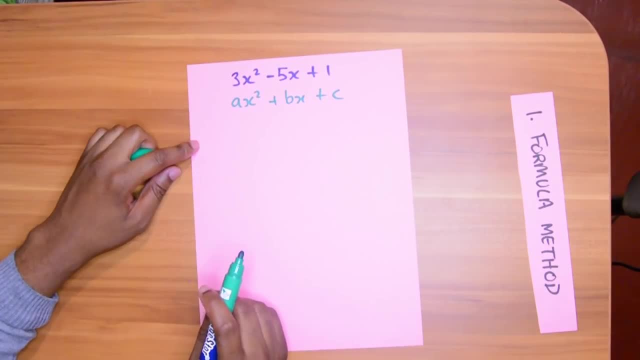 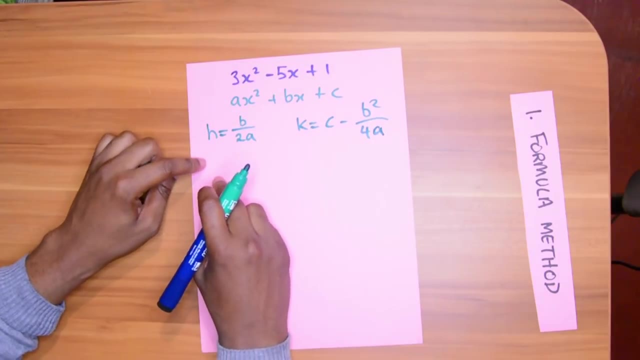 So these two guys you are using, So let's write them. Next step: write the formula and write it in the same way that I'm going to write it here. So you write H and 4A. So now that you have written the formula, all that's left to do is to plug it in and 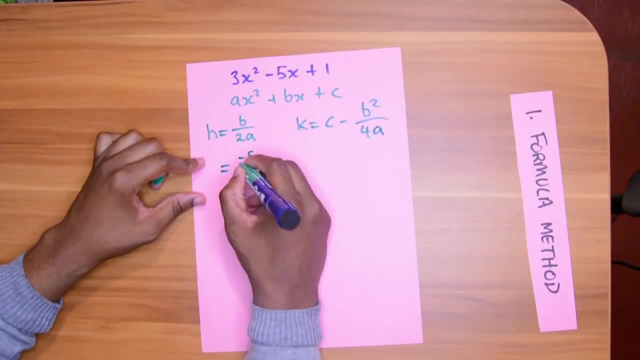 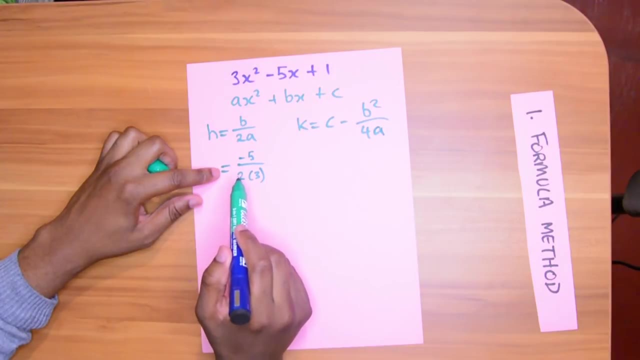 get the value. So what is B? B is negative. 5, 2 by A is 3.. So you may be tempted to plug this into your calculator and get an answer in decimals. Don't do that. Keep everything in fractions for this. 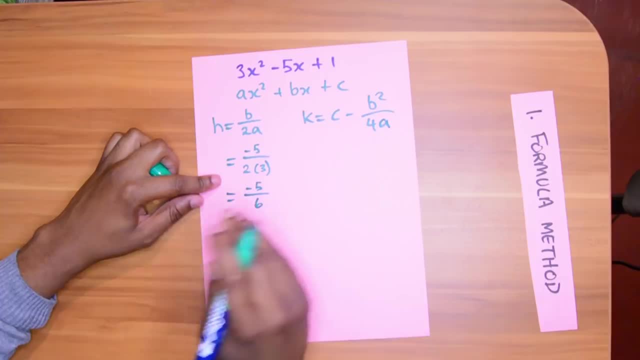 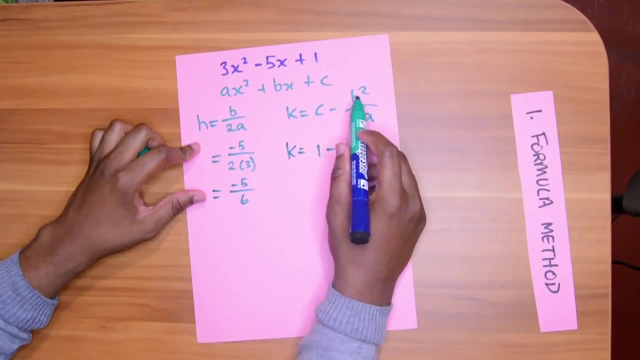 So equal negative 5 over 6.. We good with that. Fractions Beautiful. A is equal to 5.. So that's the formula. A is equal to 1. take away: B is negative 5 to be squared. A common mistake is, when we square this, we leave the negative. 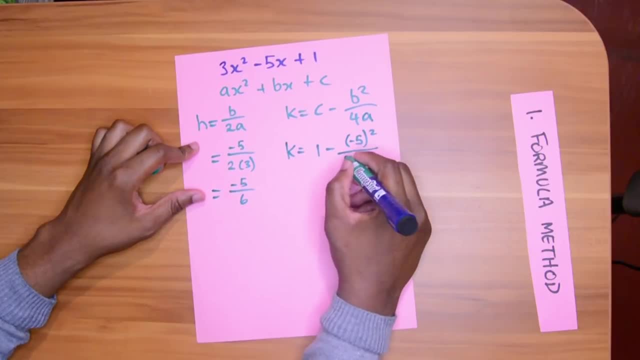 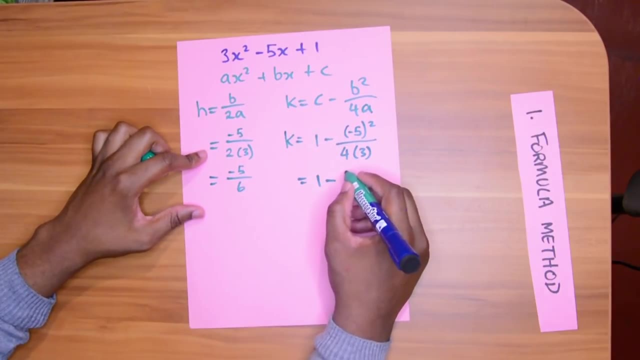 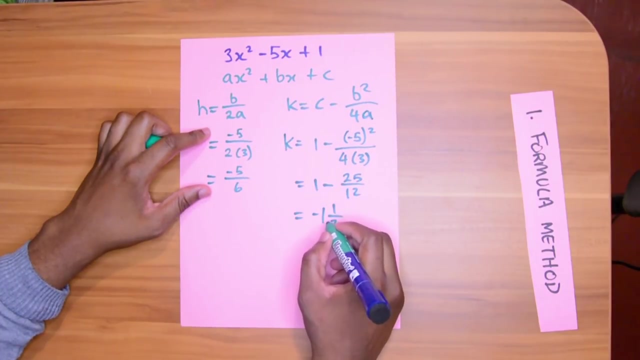 But when you square a negative number it should turn into positive 4 and A is 3, again 1. take away 25 over 12.. This leaves us with negative 1 and not a half 1 over 12.. 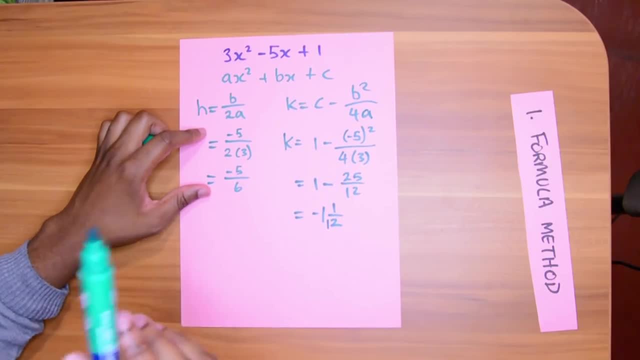 So for this part you can use your calculator, But remember to keep it in fractions or use the fractions setting on your calculator. Alright, and be careful with grouping up everything into one and solving it on your calculator. Remember to use brackets if you're about to do that, or try it part by part. 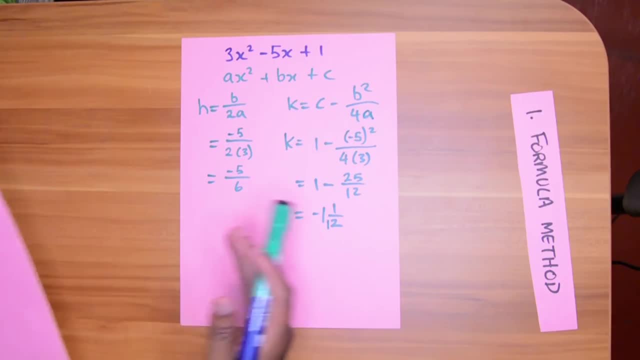 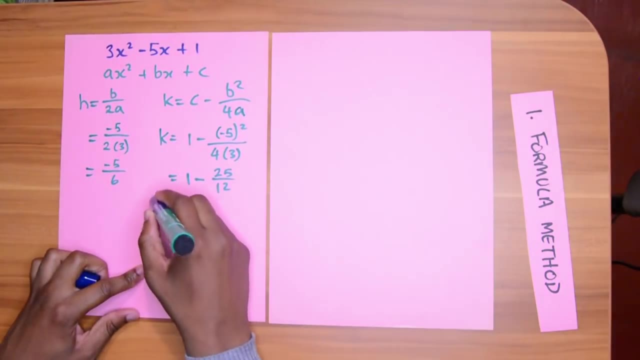 I'm telling you the common mistakes that happen. Alright, so we've practically finished here. All that's left is to actually use the values, because this here is our value for K and this here is our value for H, So we just need to use these values. 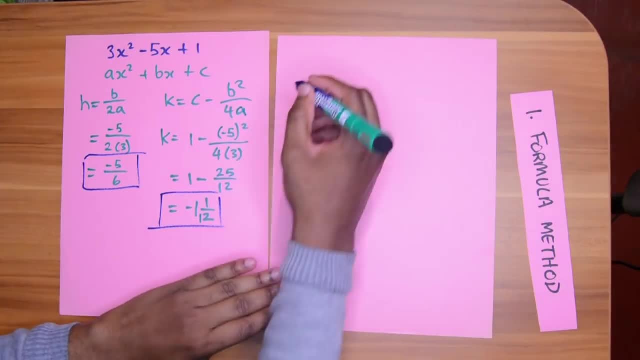 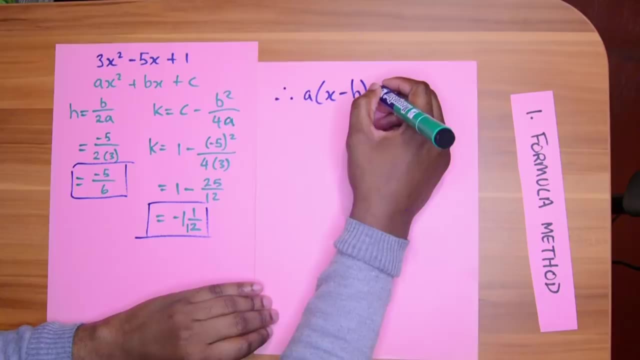 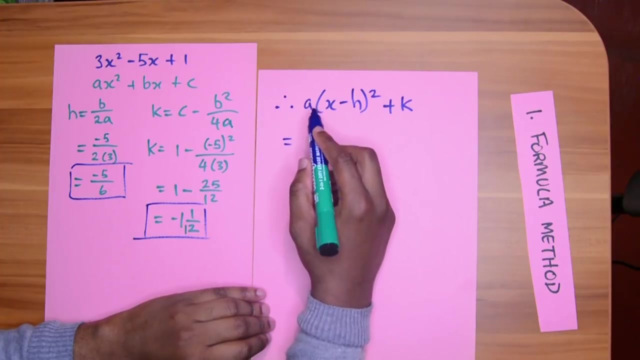 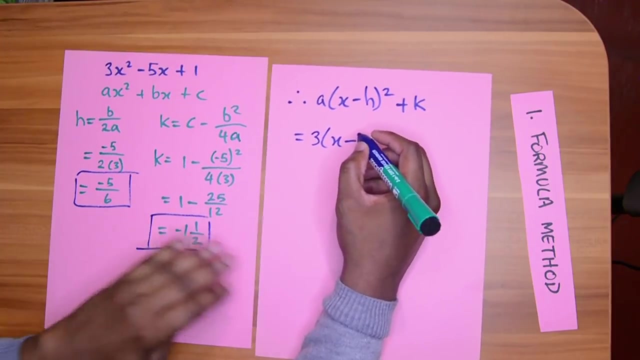 In the completed D square form. So we write therefore A into X, minus H, to be squared plus K is equal to, and we begin to substitute values: A is 3.. X, take away. H is negative 5 and 6. Negative 5 and 6.. 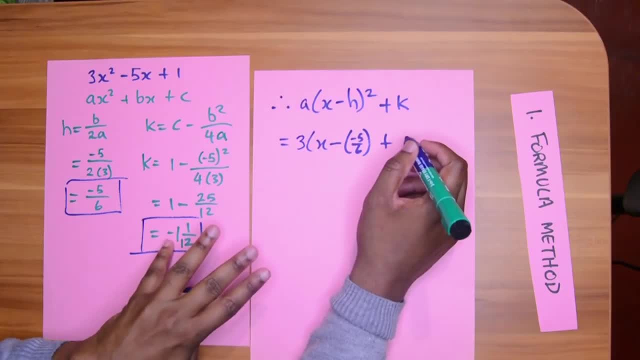 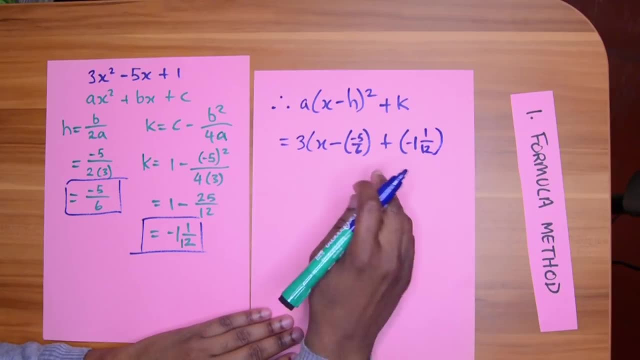 Plus K. K is negative: 1 and 1 twelfth, Negative: 1 and 1: twelfth. So it's especially important to use brackets when we are putting in values, especially if they are negative. Okay, so we just simplify 3 by X. 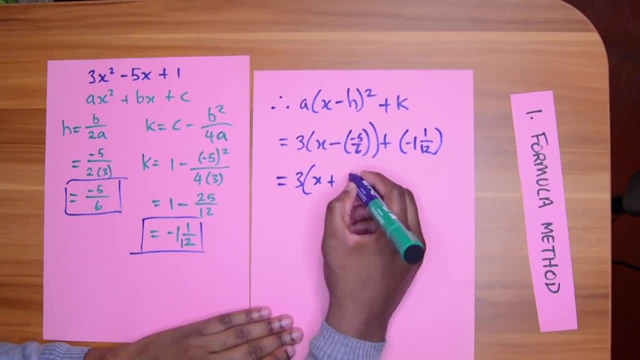 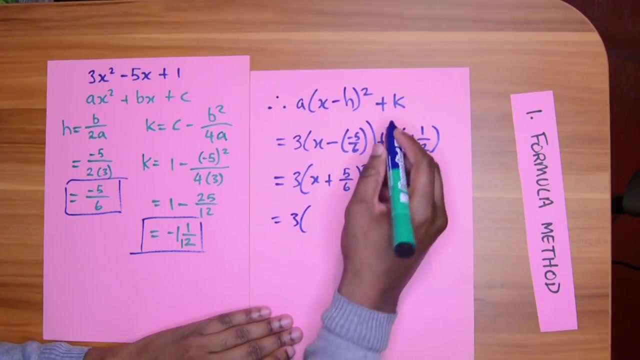 Negative and a negative. Two negative signs next to each other, And I should have simplified this sign one time. Okay, I'm going to do an extra line because I was hurry 3.. There should be a square here and a square there. 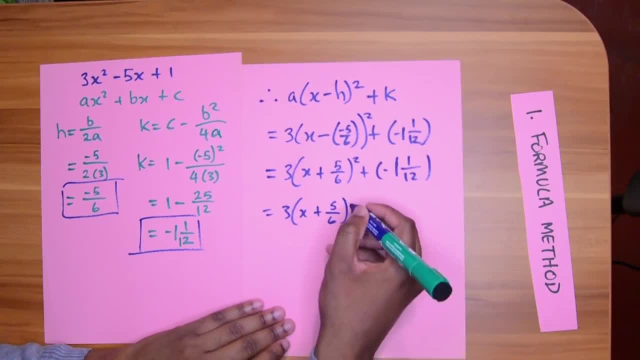 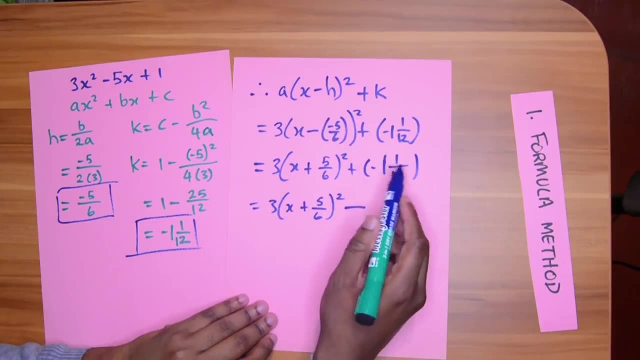 X. Don't forget there's a square there. That's a common mistake- X plus 5 and 6.. I'm changing this to 1 subtraction sign because positive and negative. What am I doing my people? And this is the answer to the question. 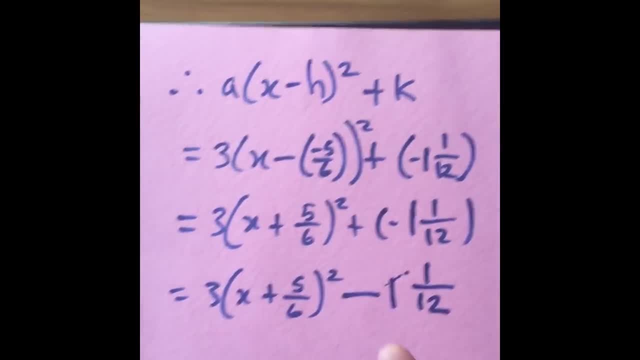 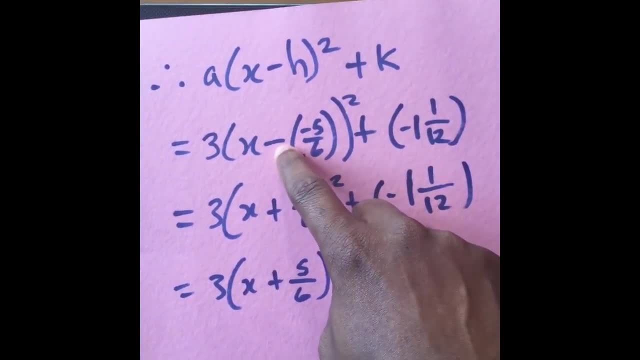 Thank you, Not quite the answer, actually. I made a mistake. I come home and I'm out checking the video And thanks to the people who sent me the mistake. This was supposed to be positive. This is positive. This would be negative. 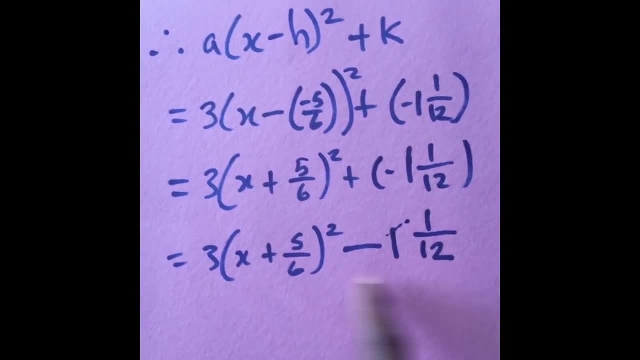 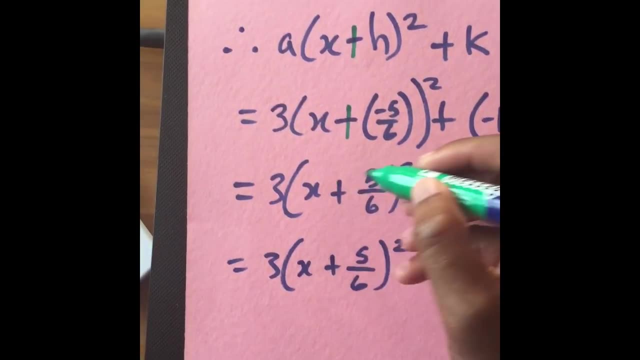 This would be negative And if you watch at the end of the video you'll see this will be the answer. we got in the last method that we do, So let me just fix that. This should be positive. This should be negative. This should be positive. 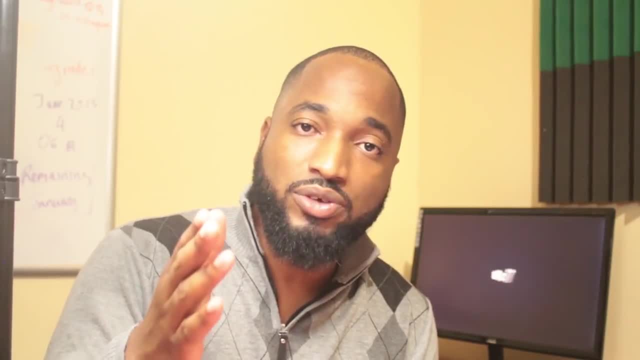 This should be negative, This should be positive, This should be negative, And I'll give you some questions to try at the end of the video. So hang on right. But first I want to do the actual completing the square method, which is method 2.. 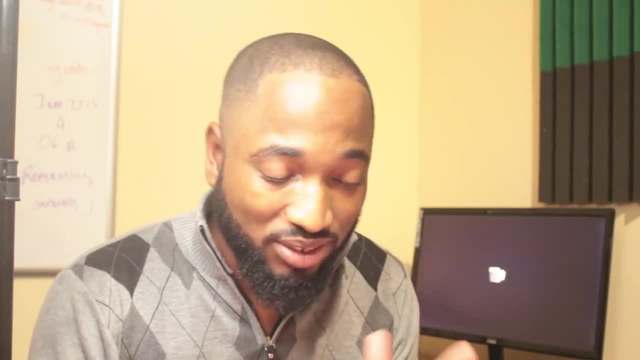 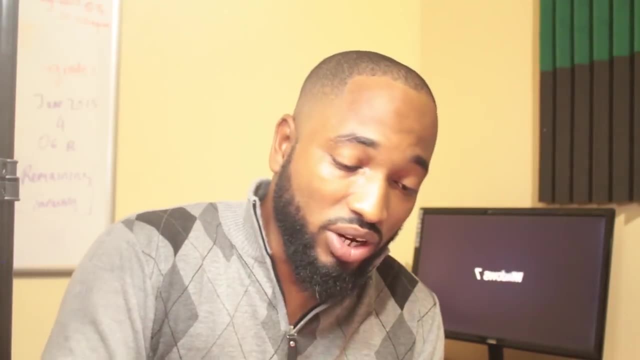 You see, the one problem with this first method is that you can actually lose or drop a mark, One mark- Because, depending on how the question is phrased, you didn't actually complete the square. You use a formula and you just simply plug in values for h and k. 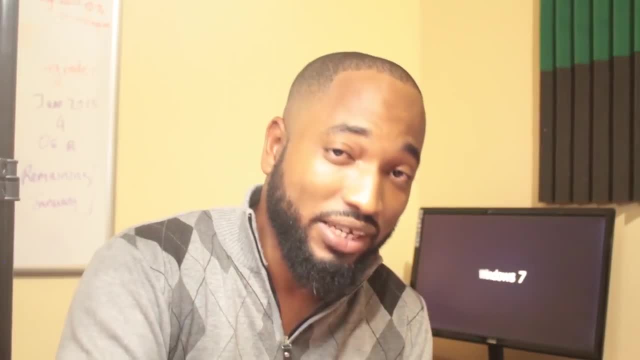 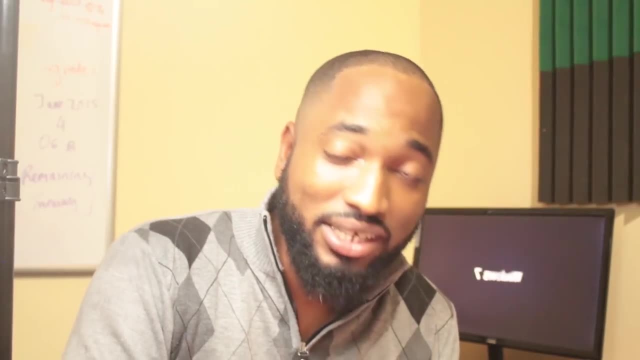 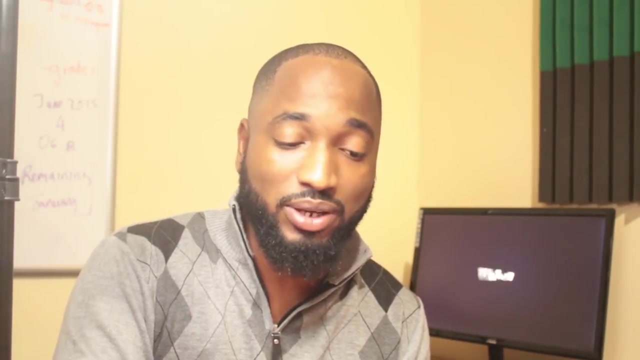 So if they said, by completing the square or by finding the perfect square, there is a possibility that you lose a mark, But it's still important to know this method because it's so easy and sometimes you might just need to do this And it's better you lose one mark than you lose the whole 7 marks for the question, because 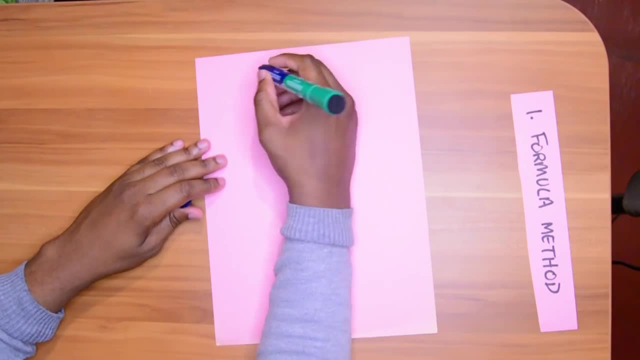 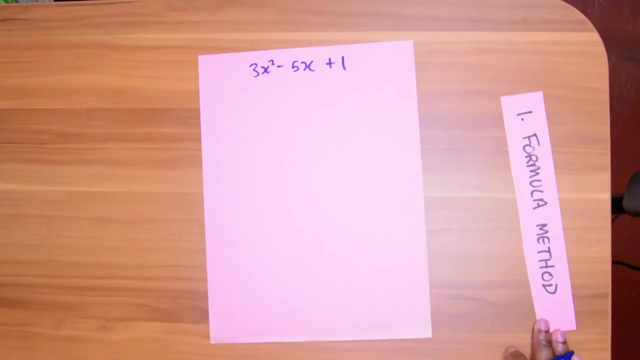 you couldn't complete the square in the first place, So let's use the same equation: 3x squared minus 5x plus 1.. This is not the formula method. This is our natural completing the square method. So 3x squared minus 5x plus 1.. 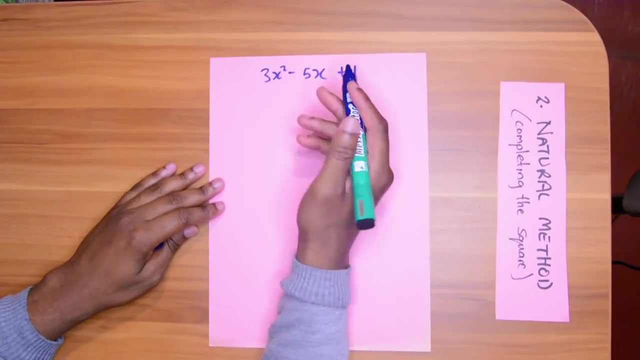 The first thing you want to do is take out a, Factorize a. Now some teachers will say: factorize a from all three terms and some will say factorize it from the two terms. I prefer to factorize it from the first two terms. 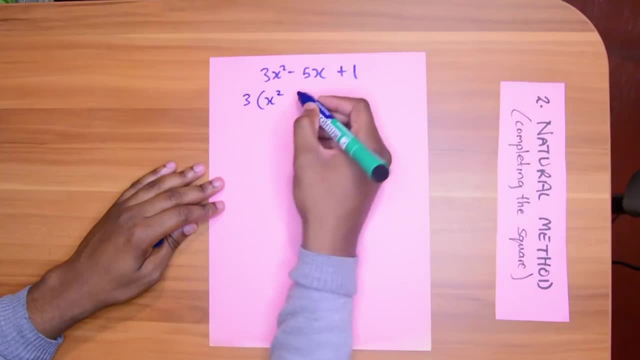 So 3x squared. take away. If I take 3 out of this, this 5 should come over 3 plus 1.. Or you can put the whole thing over 3.. But since we're just dealing with the coefficients, 5 over 3, right. 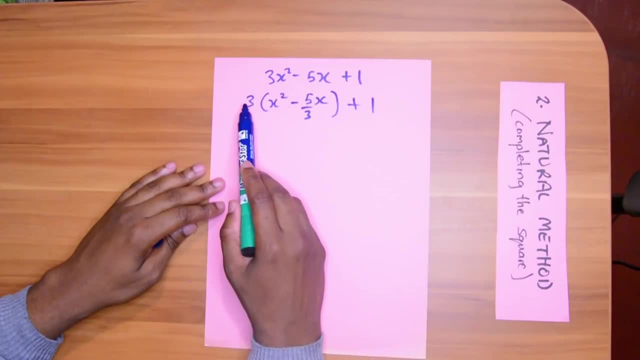 So hopefully you caught what happened there. If I multiply 3 by x squared, I'll get that back. 3 by this, I'll get that back. Alright, so we're going good so far. What's next is a kind of Jedi mind trick. 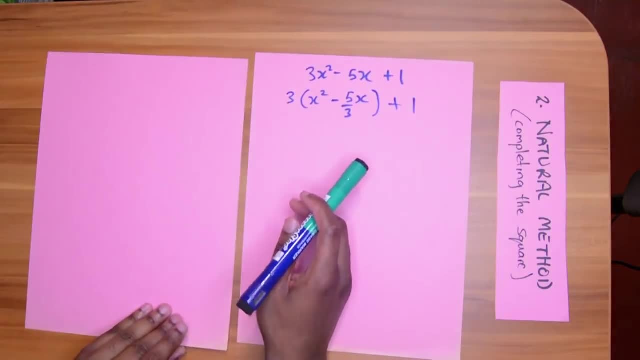 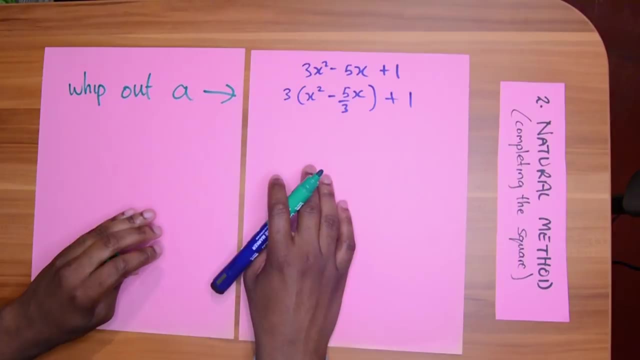 Alright. so the first thing we did, The first thing we did was rip out e. So that's the first thing we did: We ripped out the e. There's a next step here, But before you go to the next step, I want to jump that step. 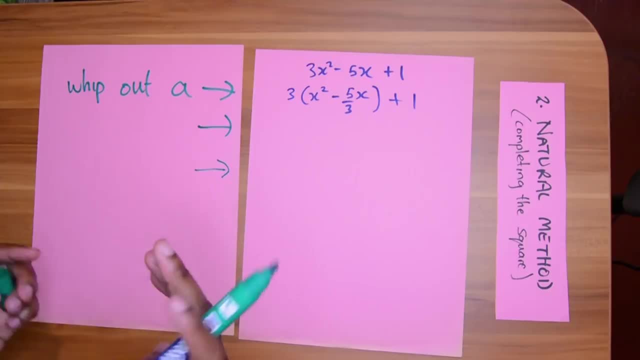 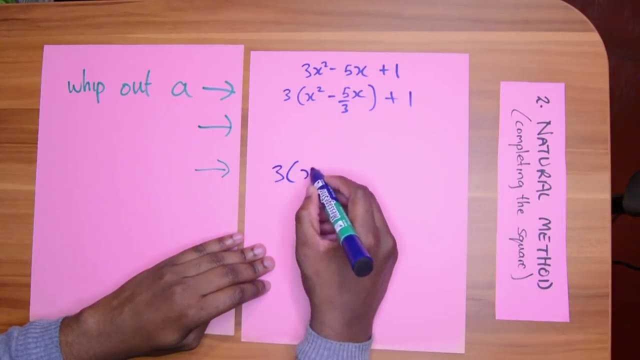 Jump that step and go to this step, Because I just want to help you understand the process. So remember, we're skipping that intermediate step. You put 3.. And now you put x, Not x squared. Take away half of this number. 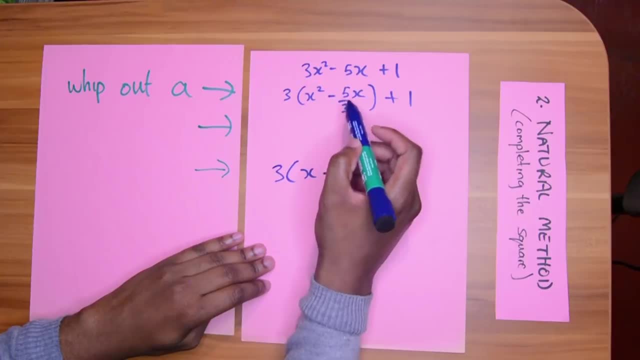 Which is 5 over 3.. Half of the 5 over 3.. Now, remember this is not a 5 here, This is 5 over e. So you want half of that number, 5 over 6.. How did I get 6?? 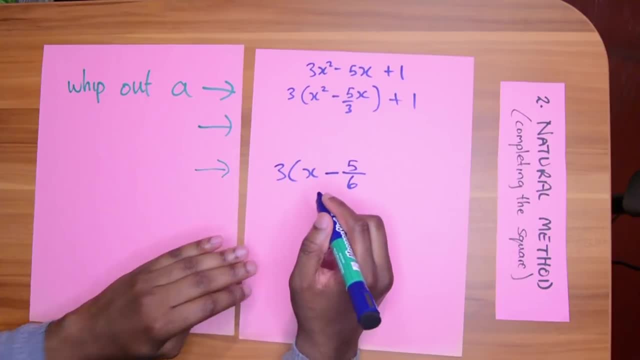 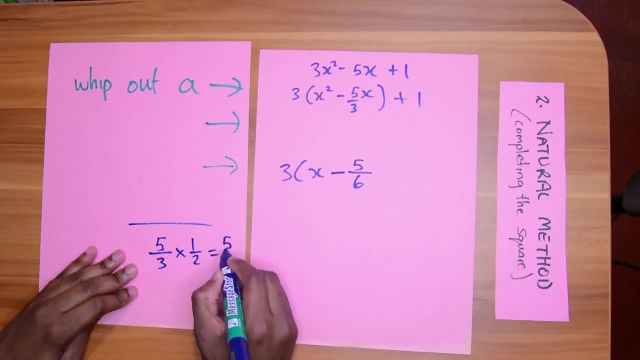 Half of 5 over 3. Is 5 over 3.. Watch the scrap here: 5 over 3. Half of that Is actually 5 over 6.. So this is a technique you can learn for completing the square. 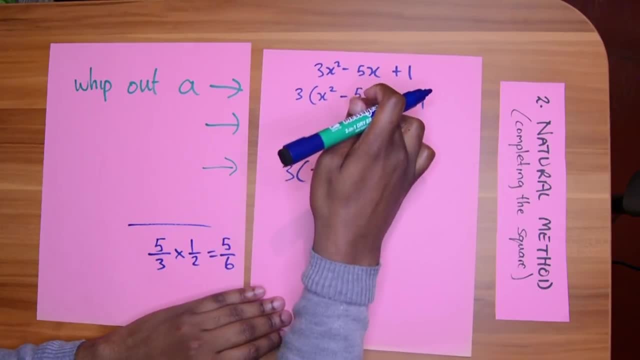 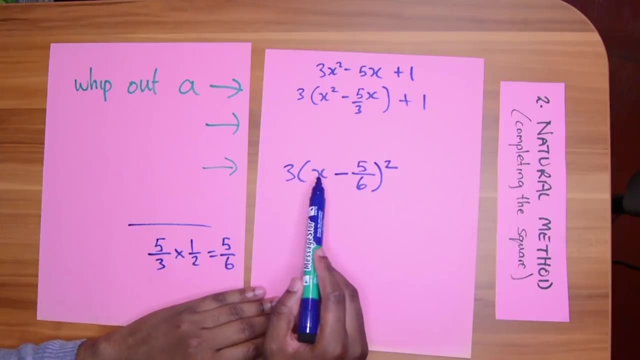 Half of, Because you'll always have to find half of this number. Close the brackets and square it. So once again, 3 by x, Not x squared. The squared comes here: x minus 5 over 6.. To be squared: 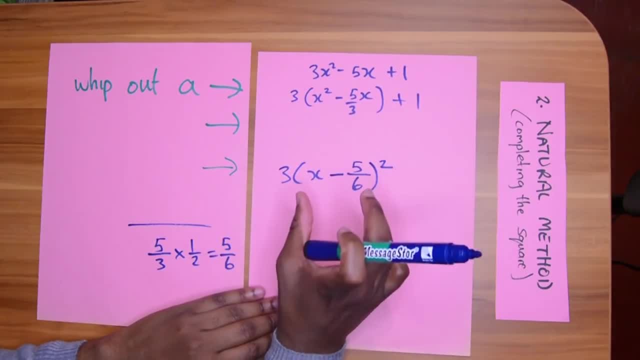 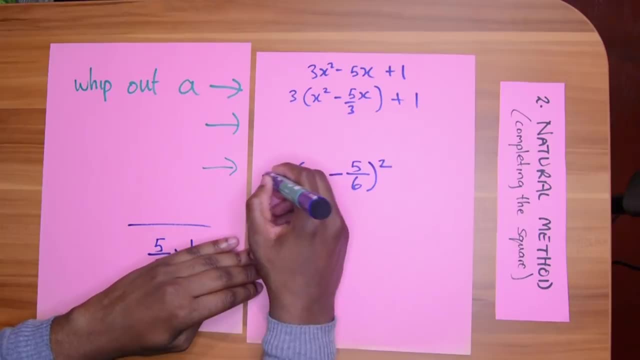 What we just did there Is create a perfect square. This is a perfect square: x minus 5 over 6.. To be squared Based on half the value of this, And that's How we complete the square. That's the key step in completing the square. 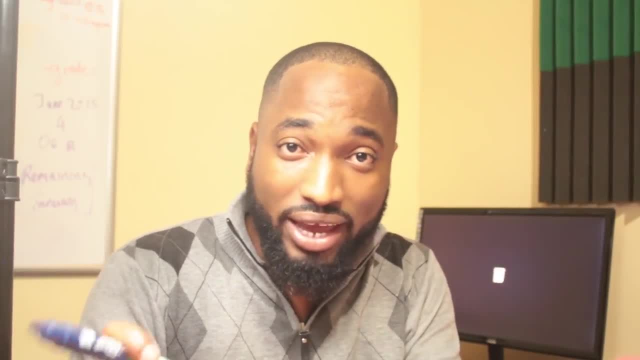 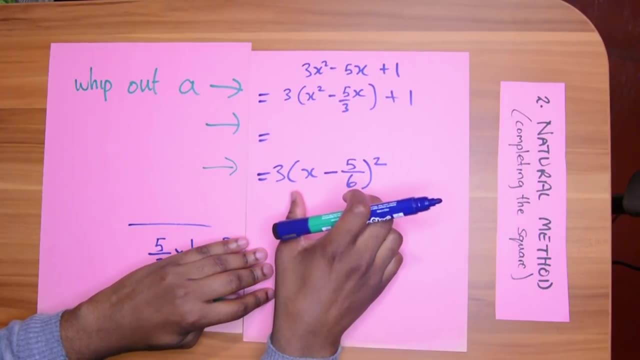 Creating this perfect square. But when you create this perfect square- This is the key part- Pay attention: When you create this perfect square, You created an extra number. If you square back out this, You would see That you get this and this. 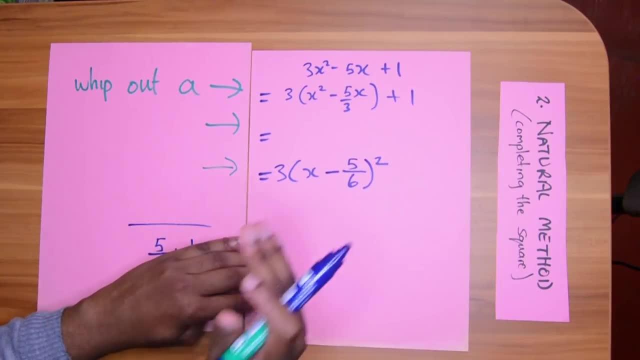 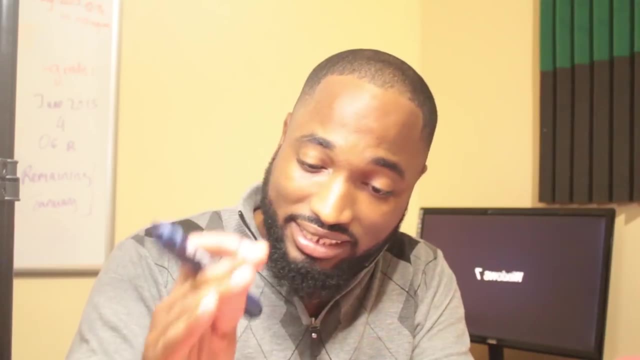 But you also get an extra number. Is This To be squared? 5 over 6.. Squared, That is the important part: 5 over 6 squared, So that number 5 over 6 to be squared. 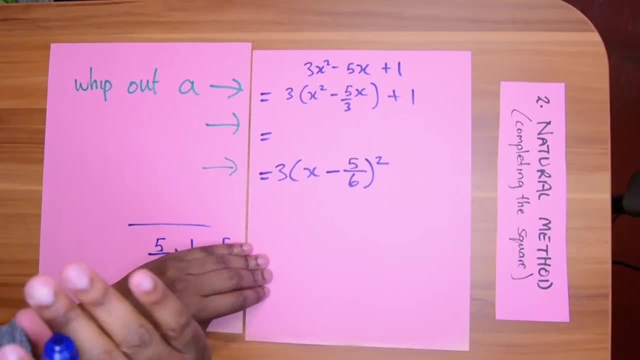 Negative 5 over 6 to be squared Must be accounted for. Now let's see what happens in this step before. I'm not finished here, But let's see what's happening here: 3. Into x squared Minus 5 over 3.. 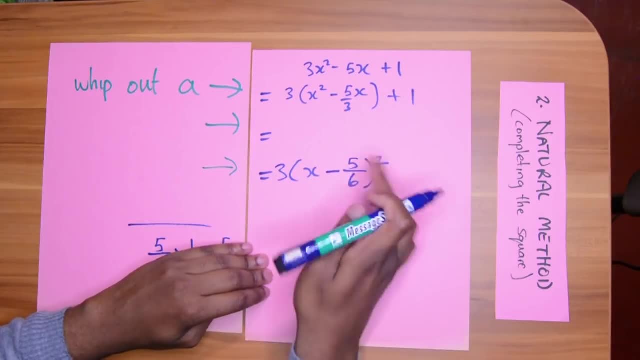 x. I'm going to put in The number that we Known as X. So I'm going to put in The number That we Known as X: X. The number that we Know Is missing. 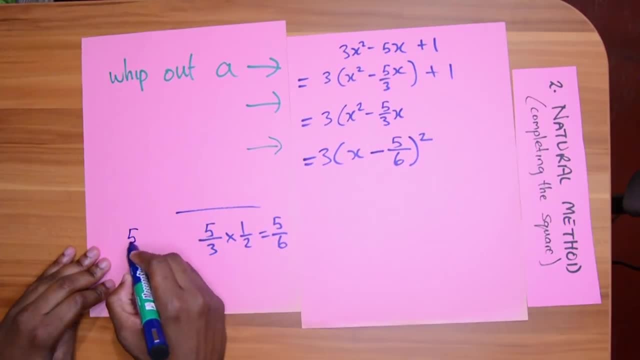 It's going to be 5 over 6 to be squared Now, 5 over 6.. To be squared Negative Doesn't matter, Because you're squaring it. It's going to be 25. Over 36.. 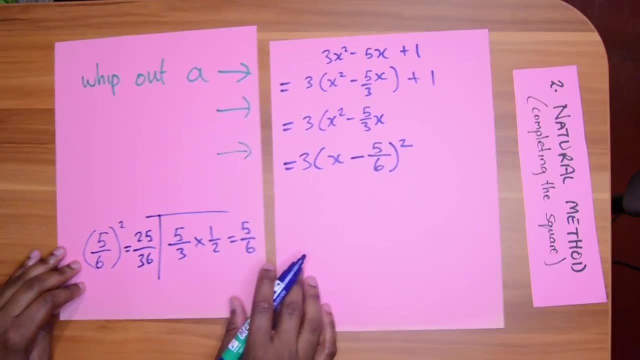 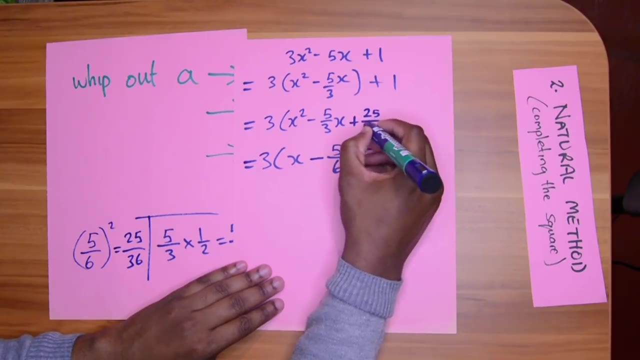 Right, So that's an extra book in there. Um, So I'm adding in 25.. Over 36. And that's the key. Put back the 1. Coming down here, So I'm adding in 25.. 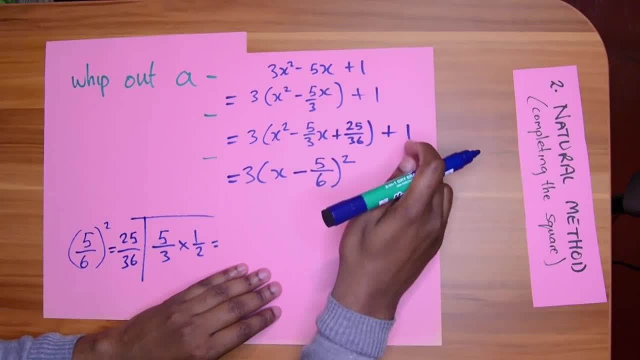 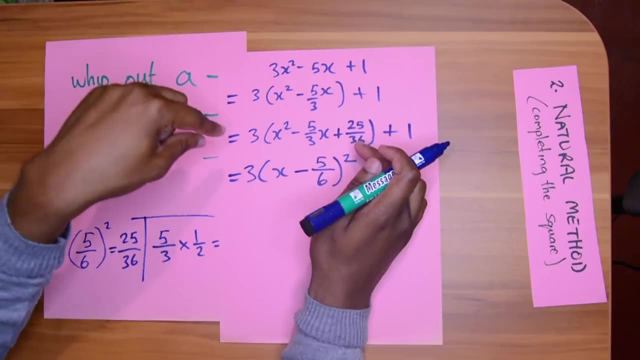 Over 36. And that's the key: Put back the 1. Coming down here. So now That we add in 25. Over 36. There's one more game This complete In the square Wants to play on us. 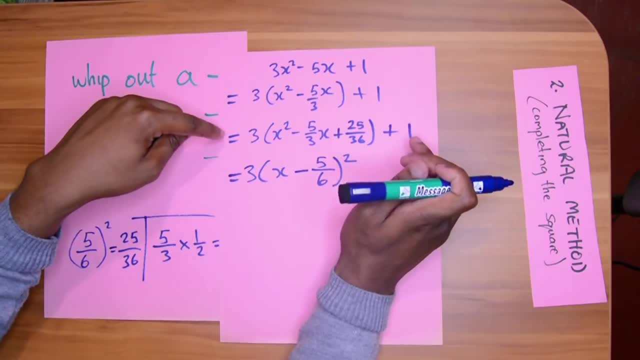 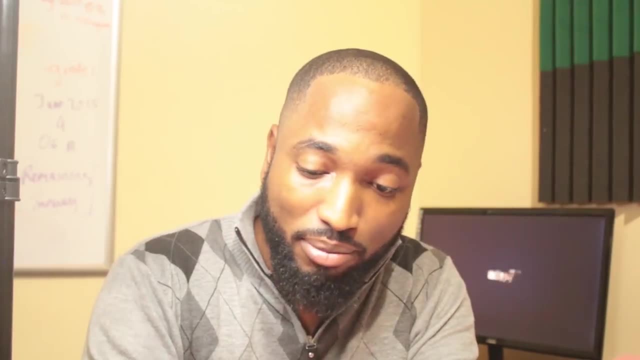 We must Multiply this 3. By the 25. Over 36. And subtract it From the equation, Because That's the only way This is going to be Equal to this. Imagine, If you're just. 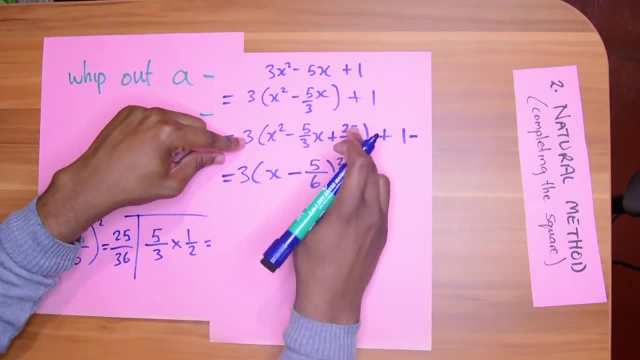 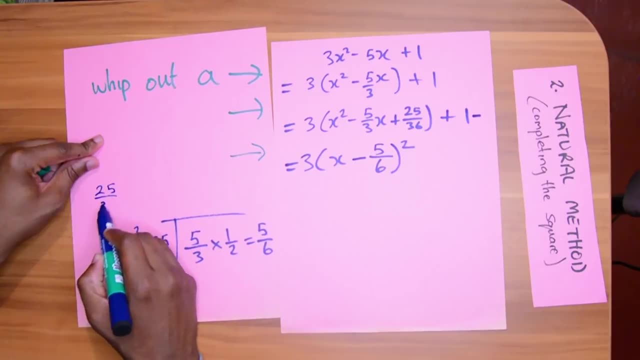 Adding a number To the equation. You must Compensate By taking All that number. But this number, Where Can I fit this? Let's fit it here: 25.. Over 36. Multiplied by 3.. 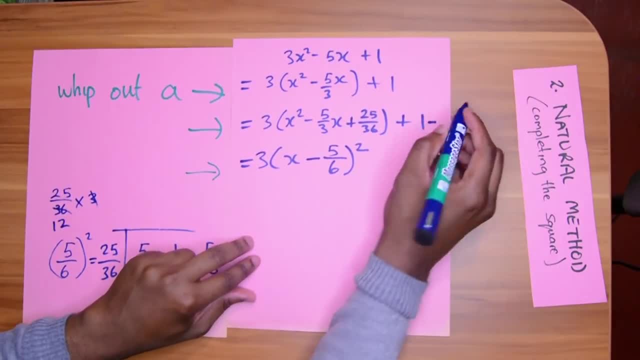 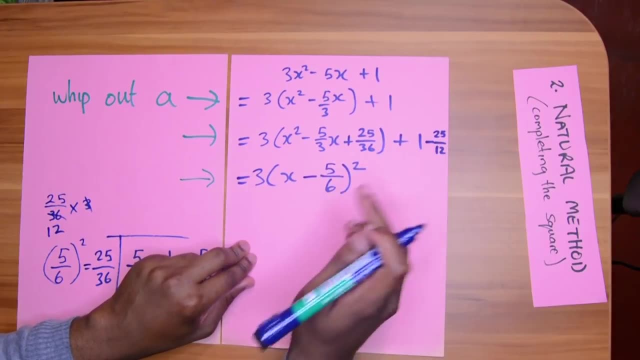 Is 25. Over 12.. So We have 25. Over 12.. Squeezing out Of the equation, So this is subtract 25. Over 12.. So one Take away 25.. 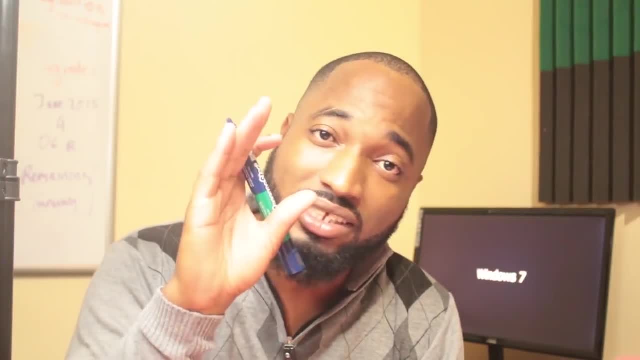 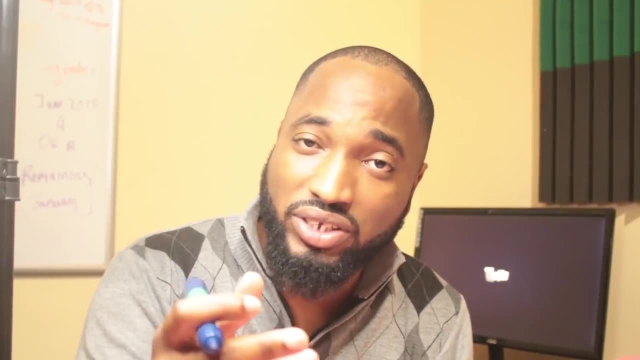 Over 12.. Now You may Need To watch That segment Several times. Do a few questions. Do a few questions, Maybe a little more Than a few questions, And you'll begin To see the pattern Easy. 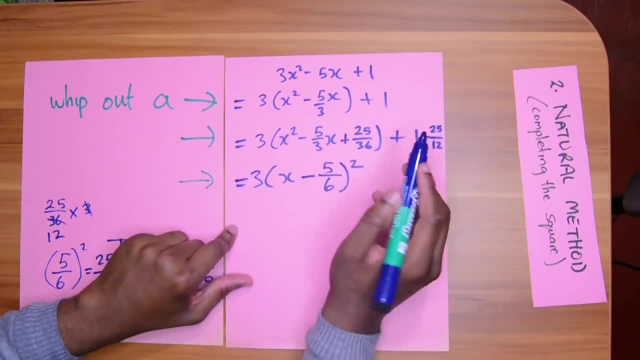 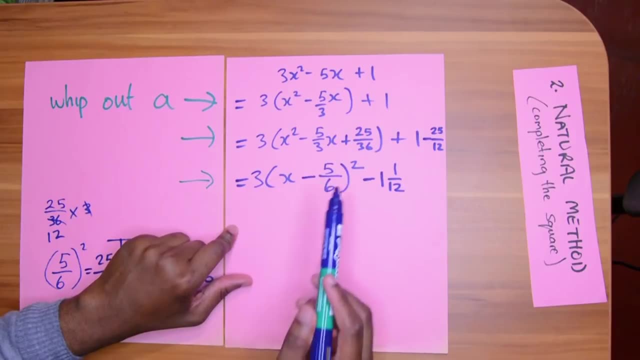 Alright. So the last Thing to do Is one: take away 25. Over 12. It's Negative 1. Over 1. 12. So once again, We kept Everything In fractions Or mixed.